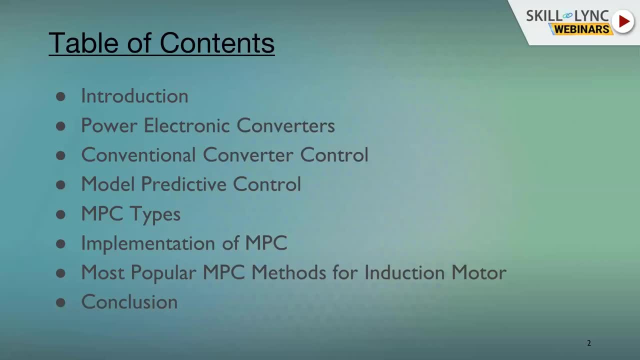 methods. Then we'll see an introduction about the model predictive control, its main stages of its development, Development or implementation, then the types of model predictive controls that are available in the literature And we take an example and see how the implementation of a model 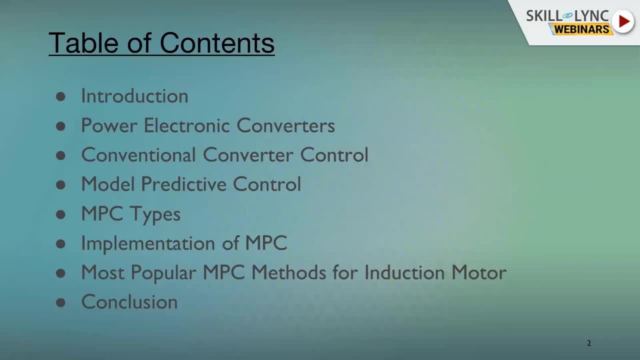 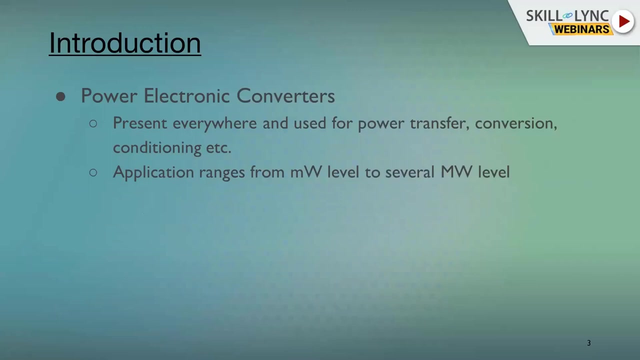 predictive control is done for a simple power electronic converter, And then we'll see two most popular MPC methods for the control of induction machine. And then we'll conclude the webinar. So introduction. coming to the introduction, we have normally seen many power electronic converters. 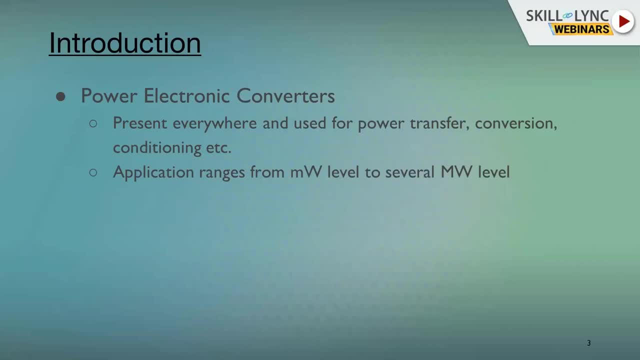 So what are power electronic converters Typically? by definition, a power electronic converter is an electronic circuit that mainly uses electronic components based on semiconductor switching, which typically operates at frequencies as low as 50 or 60 hertz to as high as several kilohertz. Now these power electronic converters are present everywhere and they're useful. 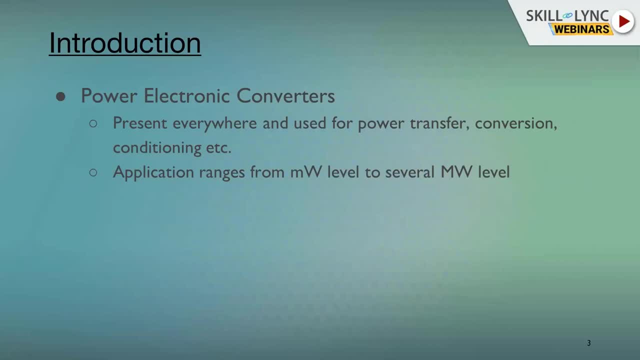 mainly for power transfer, power conversion and so on. So what are power electronic converters? Well, first of all, they're used for power conversion and power conditioning, And of course there are many more, And the applications of these power electronic converters ranges. 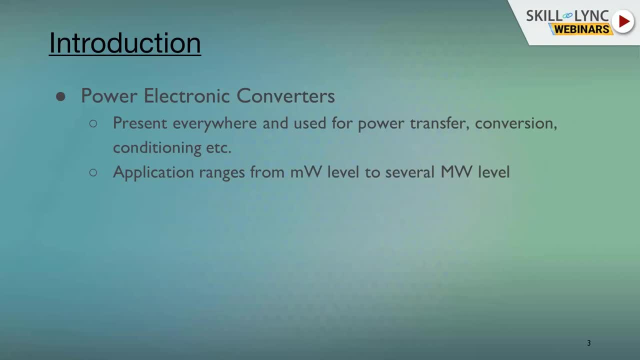 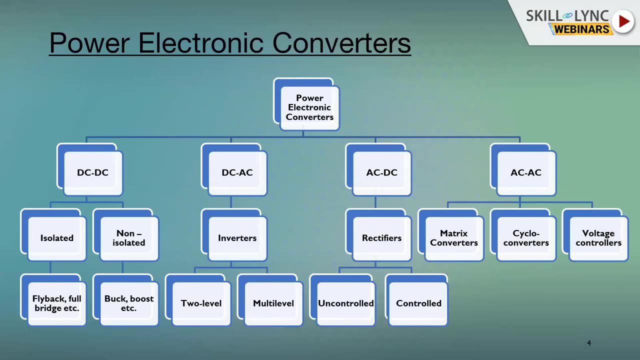 from a milliwatt range to several megawatt range. So, having said that, going to the power electronic converters and the conversions typically or broadly, the power electronic converters that are available in the literature can be classified into four categories. The first one is a DC to DC converters, The second one is DC to AC converter And the third one 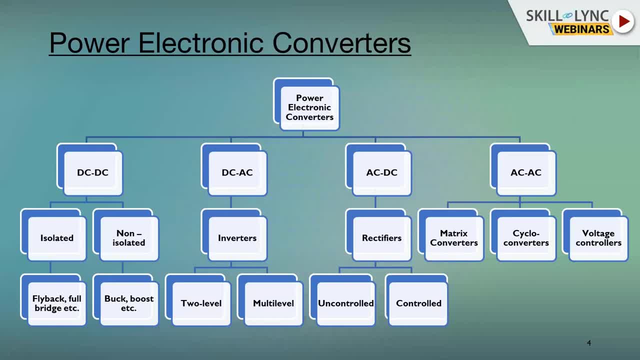 is AC to DC converter and then AC to AC converter. Now AC to DC converters are typically- again, they can be broadly again classified into isolated converters and non-isolated converters. The isolated converters are an examples for the isolated converters are fly back or a. 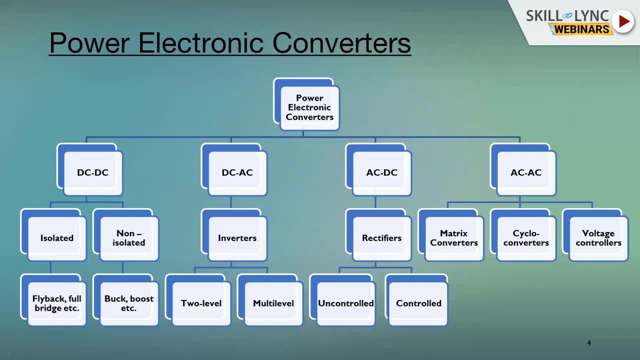 bridge converter And the most commonly used buck or boost converter is an example: forest located converted. The DC to AC converters are widely called as inverters and there are a wide variety of topologies that are available in the literature, ranging from single-phase circuits to three-phase. 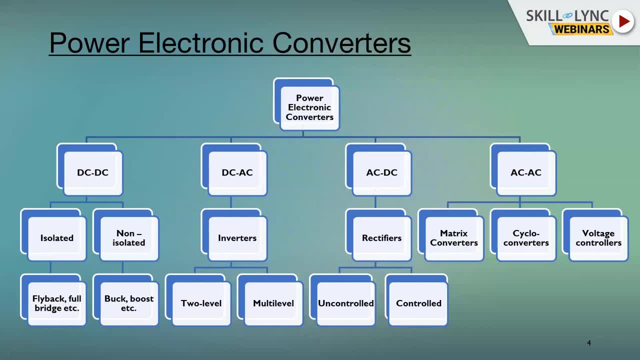 circuits and from two-level inverters to multi-level inverters. AC to DC converters are typically called as rectifiers, and they are again broadly classified to uncontrolled rectifiers, which are mainly using diodes, and controlled rectifiers that use active switches. AC to AC converters are again typical examples of AC to AC converters are matrix converters. 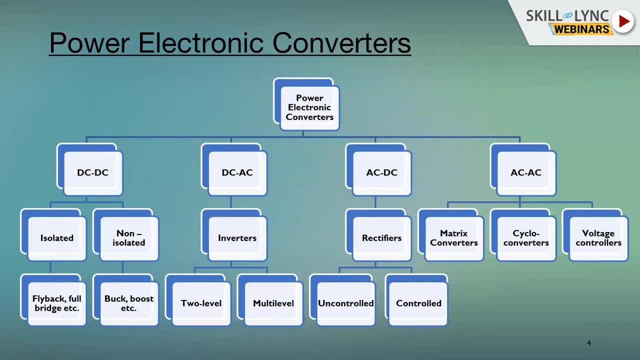 cyclo converters and AC voltage converters. Now, all these converters, as I have mentioned earlier, they are mainly used for power transfer, power conditioning and power conditioning. So let us see some examples of most widely seen power electronic converters in our day to day life. 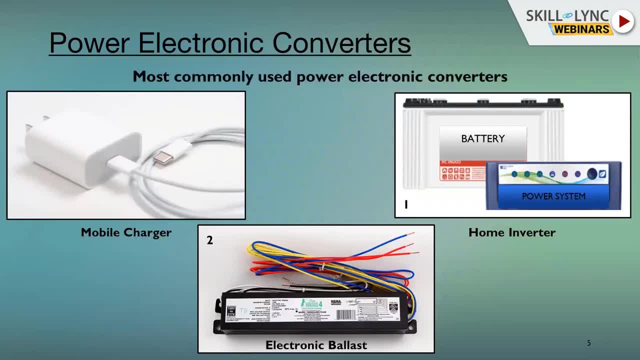 So the first one is the most widely seen power electronic converter that we encounter on a daily basis is a mobile charger. If you take a mobile charger it actually converts a 230 volts fixed frequency AC into a DC of some somewhere around 5 to 25 watts to charge your mobile phone. 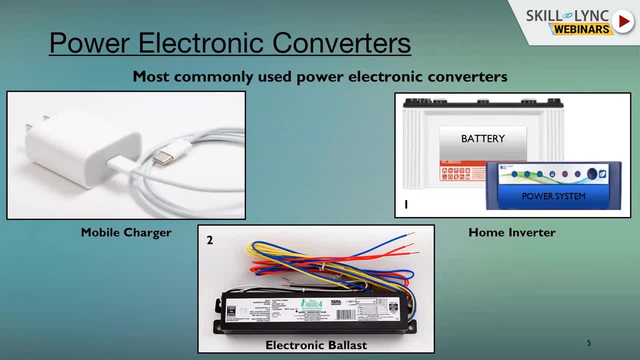 It typically employs an uncontrolled rectifier with a flyback. Another widely seen power electronic converter that we encounter in our day to day life is a typical home inverter system or a UPS system. Normally we see home inverter systems that are available at our homes, which are widely. 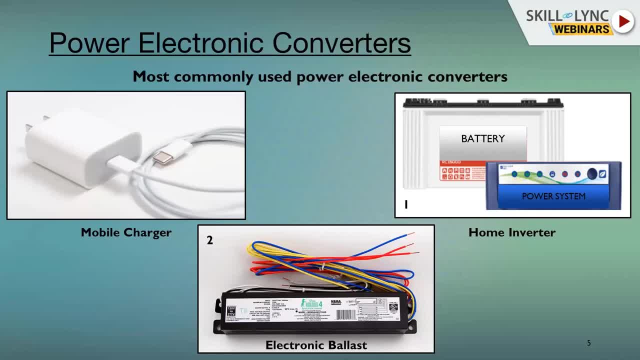 used when there is a power blackout or something. Now again, they use a simple half-bridge circuit which converts 12 volts DC to appropriate 230 volts AC. Then the third one is an electronic ballast. The electronic ballast is mainly used in the tube lights replacing the starters, and this. 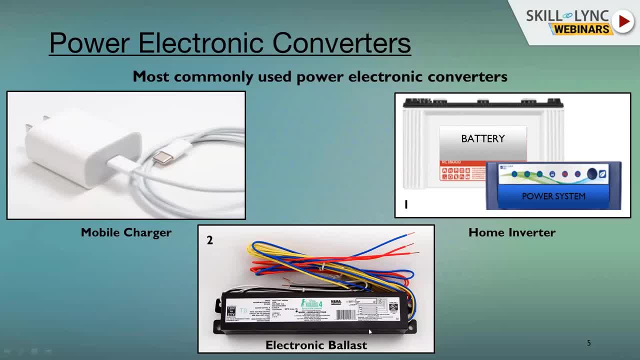 typically uses a simple, uncontrolled diode bridge with a boost power factor correction circuit. These are the typical or the most widely used converters that are that we normally encounter on a day to day basis. Now, having said this, there are certain converters which we do not use in our daily life. 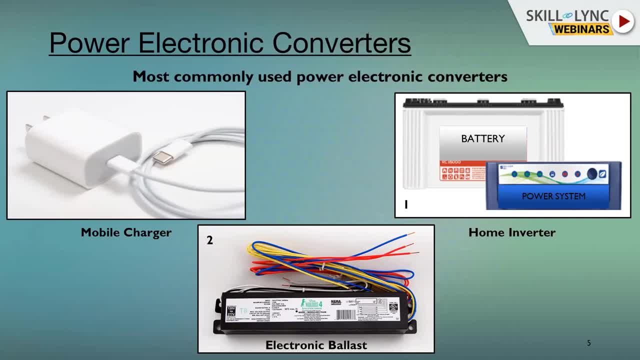 So let us take a look at some of the converters that we normally encounter on a day to day basis. Now, having said this, there are certain converters which we do not use in our daily life, So let us take a look at some of the converters which we do not use in our daily life. 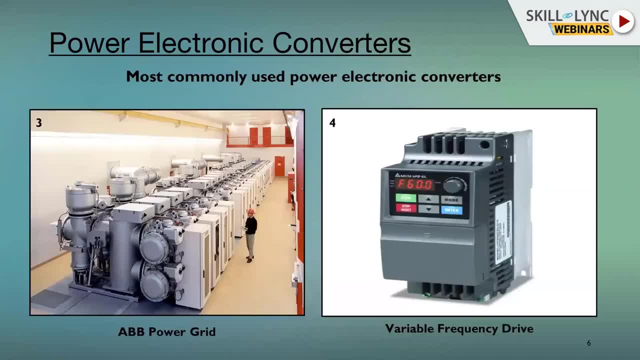 So let us take a look at some of the converters which we do not use in our daily life. So now let's see why this B servir the home internet ancient lease. This is an electronic power grid. Here is the left side picture is an example of a power grid where you can see power electronic. 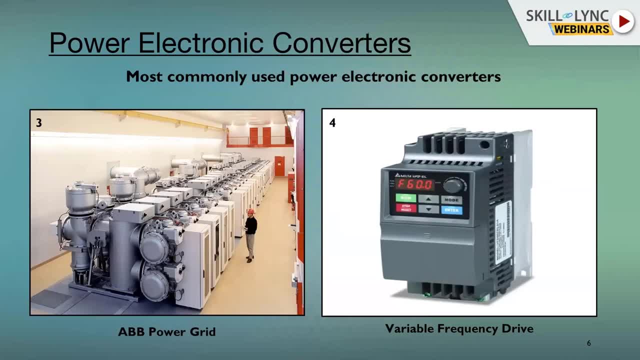 converters ranging or having of the power range of several megawatts that are connected in series, parallel, whatever. there are cascaded converters, they can be converted, they can be connected in many fashions and that are forming a complete power grid. now here they. 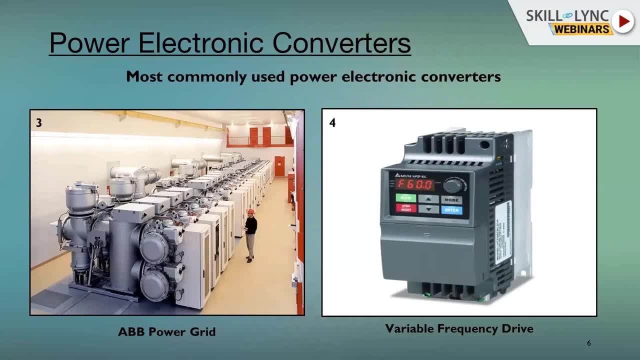 are mainly. some of the power converters are mainly used for power conditioning, for example a statcom. a statcom mainly use is used for power quality improvement or improvement of power factor or or restoring the voltage sag or swell on the power grid. now on the right side there is a variable frequency drive which is mainly used for the 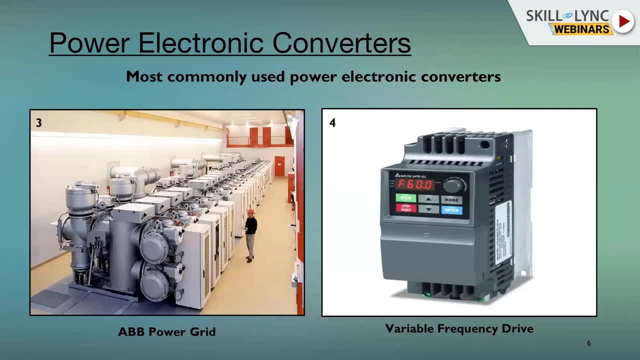 control of a motor. so a typical. these two are typical examples of power electronic converters that are industrial grade or used mainly in industries and which are not mainly used in which we don't encounter in our day-to-day life. these are some examples. there are many more uh. 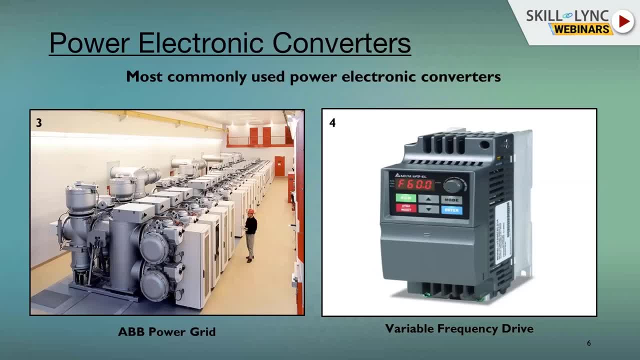 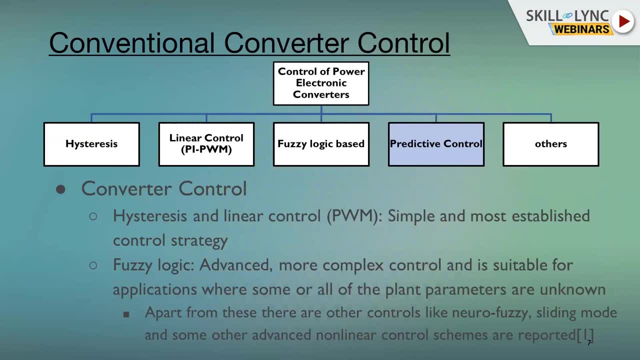 many more power electronic converters that are available. these are just some of them, which i just wanted to show you. now, coming to the conventional converter control, now the control of power electronic converters, typically in the literature there are many control mechanisms or algorithms that are reported. now some of them i have listed here, in which the first hysteresis and linear pwm controls. 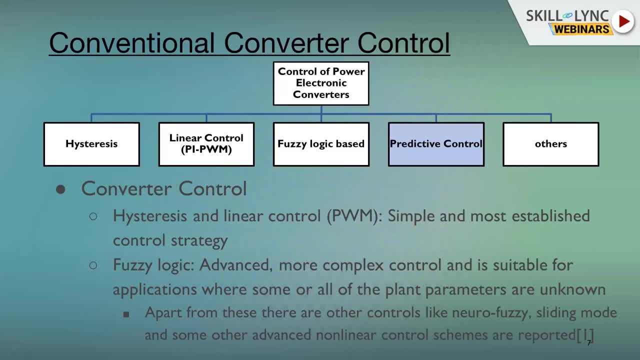 these are by far the simple and the most established controls which are mainly used in low and medium power applications and they are widely used. and there are fuzzy logic based controllers which are a little more advanced but they are little more complex in nature and is on, and they are only suitable when 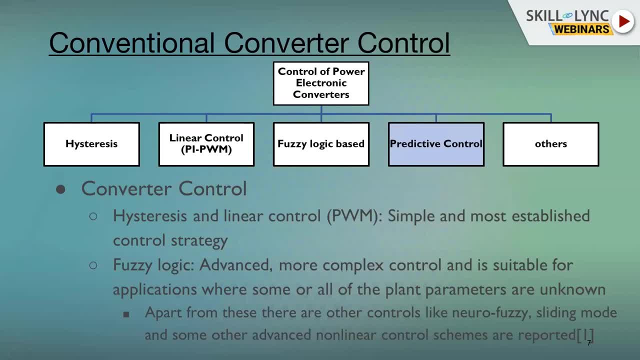 you don't have a plant information completely now. predictive control is now one of the emerging topics in this control of power electronic converters and apart from the predictive control, there are certain many other control techniques that are available in the literature, like dashdesk, using hf detective controller, neuro4z and h infinity controllers, and 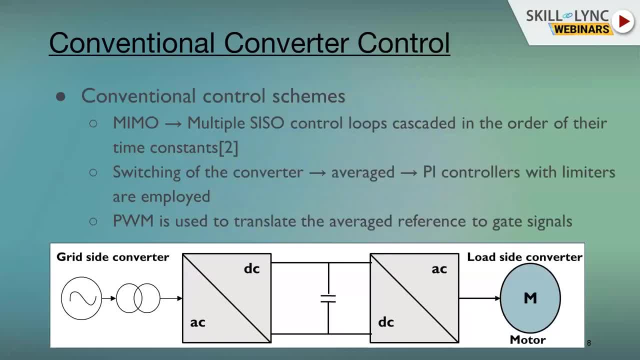 other advanced non-linear control schemes are also available in the literature. now coming to the conventional control schemes, let us take an example to understand how the conventional control schemes really work. so the below figure shows you a typical example of a variable frequency drive structure that is connected to a grid, so it has 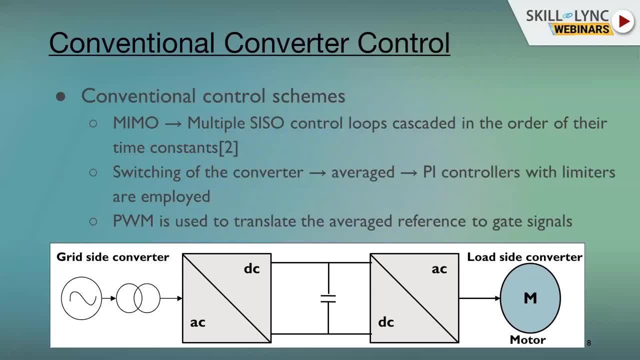 converter and DC to AC converter and with the DC. So usually all the motors normally require a variable frequency, variable voltage supply. So the typical or most widely used converter structure for a variable frequency drive is this, with where in the fixed frequency AC from the grid is converted to DC and the DC 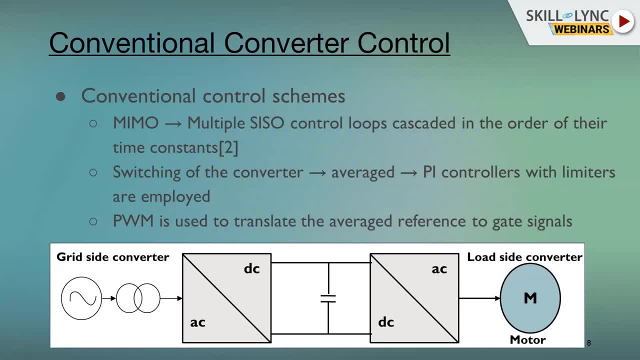 is converted to a variable frequency, AC at variable voltage. Now, in this, because the left side converter is connected to the grid, it is usually called as a grid side converter. and the right side converter is the, because it is connected onto the load- here in this case, which is a motor, it is called a load side converter. 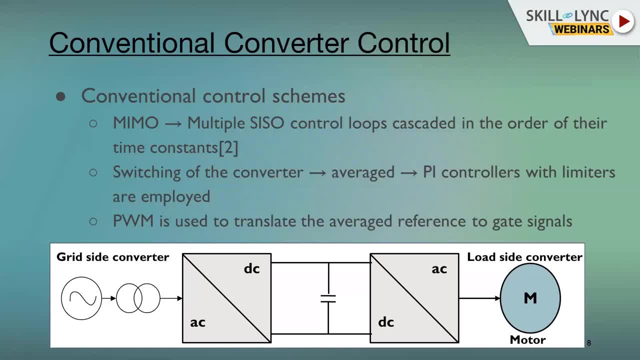 Now, adjusting the phase and amplitude of the voltage on the rectifier defines or controls the power flow from the grid to the circuit, The DC link, and similarly, here, adjusting the voltage and amplitude and the phase of the voltage of the DC to AC converter controls or enables us to control the power flow onto. 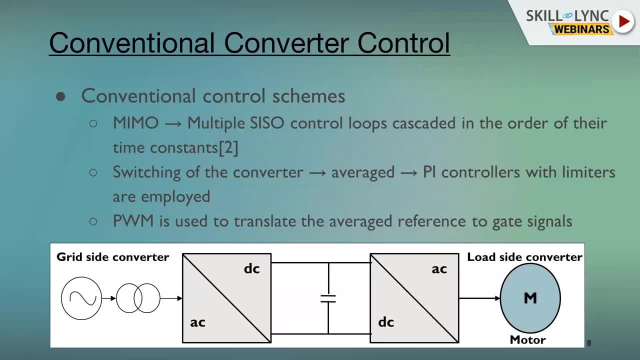 the load. So what now? coming to understanding about the requirements of a control system scheme for this, Having seen that There are three pivotal requirements for any control scheme to control this, Now one is we need to see: We need to have a lower distortions with respect to the switching losses. and then the control. 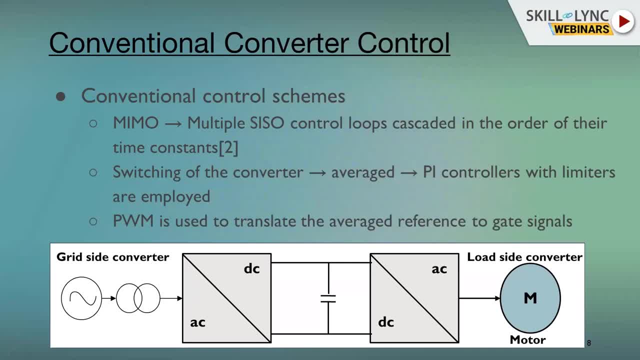 algorithm should have or should be capable of controlling the converter at a reasonably fast rate. And the third one is to have an accurate load power control. So typically the load side Converters are used or controlled in a fashion with outer speed loop with an inner current. 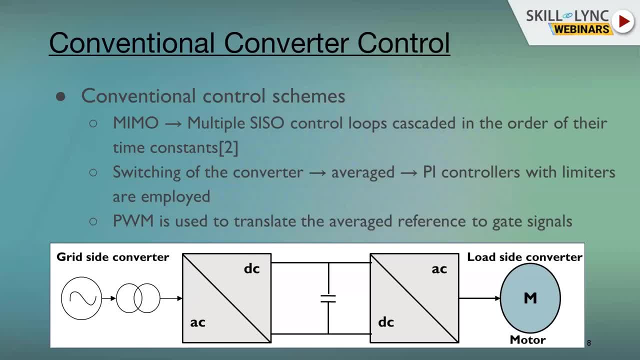 loop, So cascaded structure is implemented and the control is mainly a field oriented control with a carrier based PWM And typically the grid side converter is used with a voltage oriented control where in the peer the active power- the active power is- is taken as the reference to control the DC. 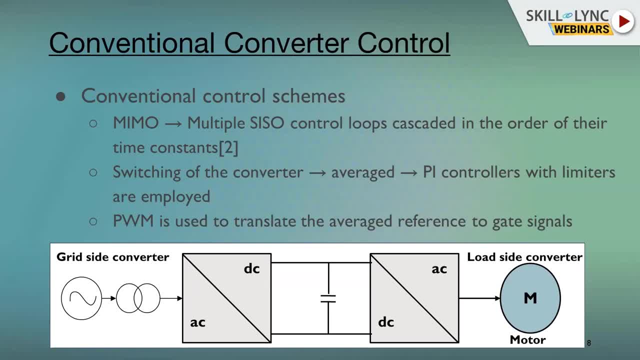 link: voltage and the reactive power is the reference, for the reactive power is kept zero. Now these? these is one sort of control mechanism. Now, another sort of control that is conventionally used is a lookup table based control, which is typically called as director control on the load on the load side converter, which 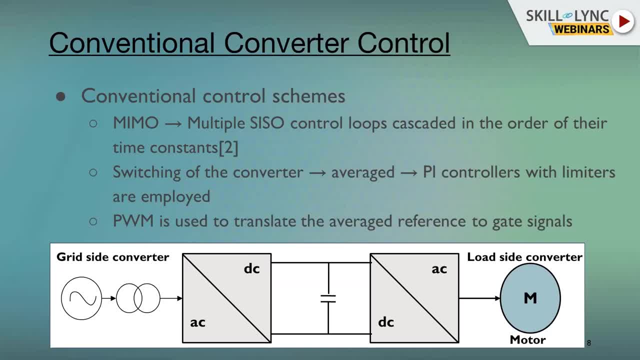 is similarly direct power control on the grid side converter. These normally use a lookup table based approach. wearing My modulator is not good to use, So the the hysteresis based control with a lookup table directly imparts the switching states onto the converters. 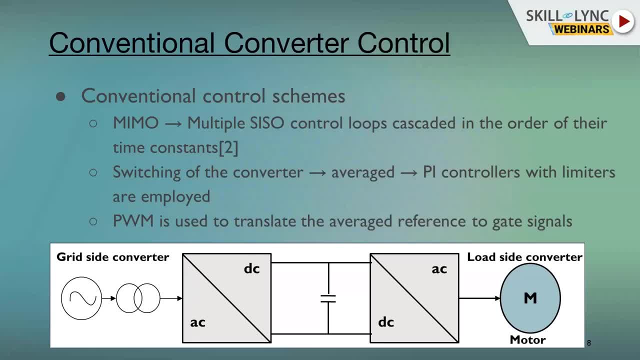 So in these methods we directly impart switching states onto the converters. They are reasonably fast, in fact very fast, But however, the distortions encountered using these methods is little higher when compared to the other methods that I just mentioned: FOC and voltage oriented controls. 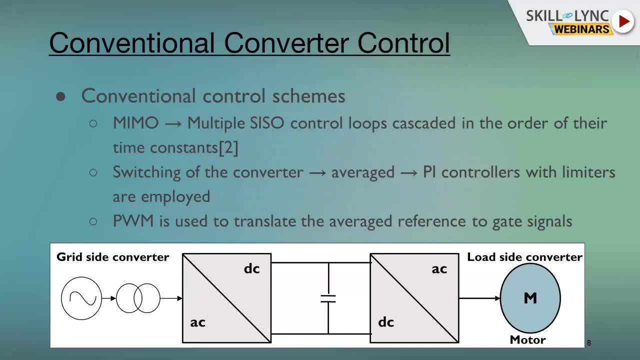 Now, apart from these, there are other methods that are mainly designed for having lower distortions. They are mainly called as optimum pulse pattern controls are a typical example of that can be taken as selective harmonic elimination is one such method which can work to reduce a particular harmonics, like, let's say, a particular, if you have a constraint on the harmonics. 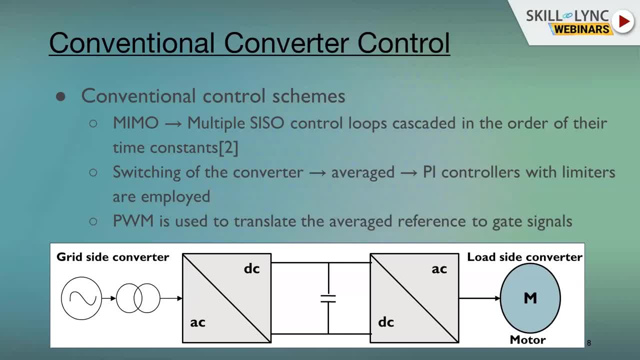 So you want some a particular harmonic to be eliminated, or you want a particular set of harmonics to be eliminated. This optimum pulse pattern controls can also be put to use in order to eliminate that kind of harmonics. The advantages with these kind of methods are they are very good in reducing the harmonic. 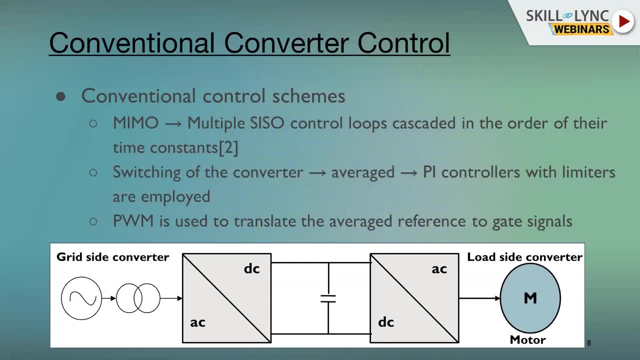 distortions. but they are very difficult in implementation, They are very slow in implementation. So typically these HEPWM Optimum pulse pattern controls are implemented only in open look with V by F kind of a control schemes for any motors. Now, having said this, after this, after looking at the multiple control systems, control methodologies, 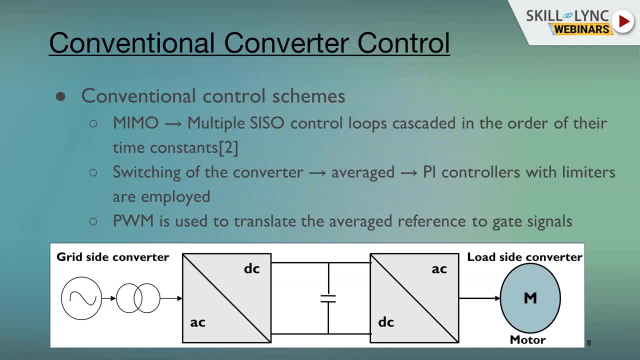 like a field oriented control, or direct or control, or direct power control or optimum pulse pattern control. These majority of the schemes. they have three attributes in common. One is, if you have a multiple input, multiple output system, All these, all these control methodologies normally convert them into multiple. 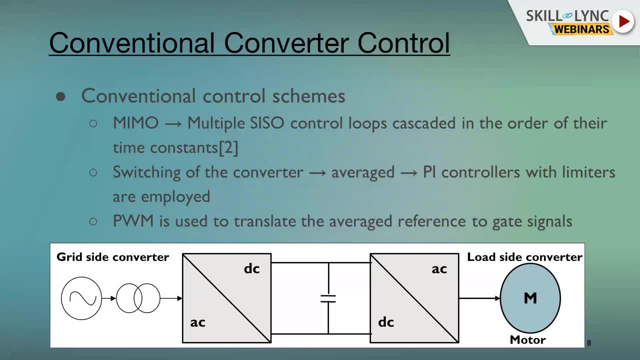 Ci. so control loops like multiple, single input, single output, control groups and they are cascaded in the order of that, Typically for any motor control. being normally put, the currents keep them on speed outside, as the speed is much slower because it is a mechanical quantity. 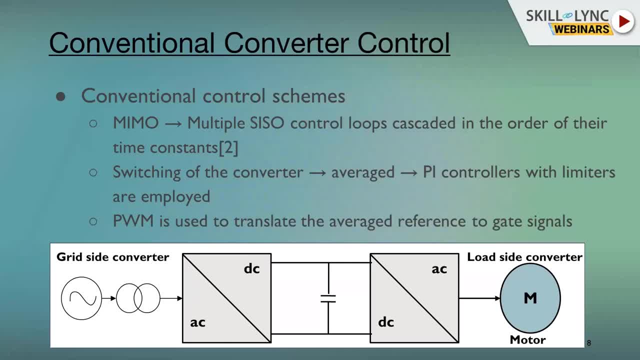 The speed is much controlled in a much slower fashion and he get the slower than the current controllers. Whereas the currents are in the time constants for the current loops are in the order of milliseconds, whereas the time constants for the order of the control of the speeds will. 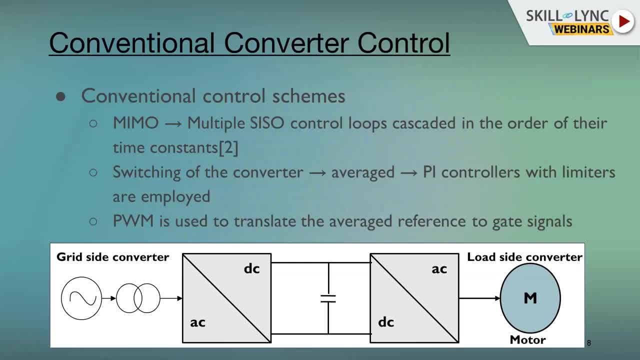 be in the order of seconds. So inner current loop and outer speed loops are typically used for multi-input, multi-output control. Then one of the another attribute that we normally see with the conventional control methods is the switching of the converter is always neglected. 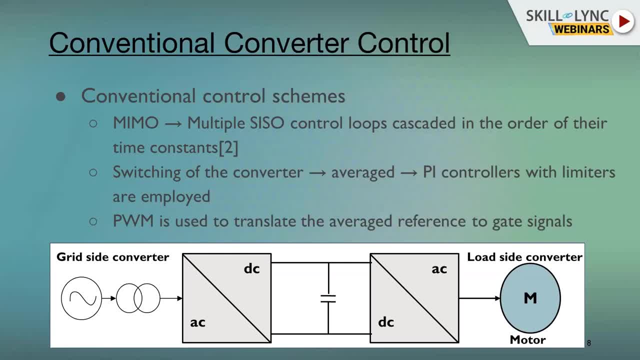 Like we normally take, the power flow from the grid side to the load side is happening only due to the fundamental component. So the moment we take the fundamental component, all the harmonic components are normally neglected, or the power flow happening with the harmonic components is normally neglected. 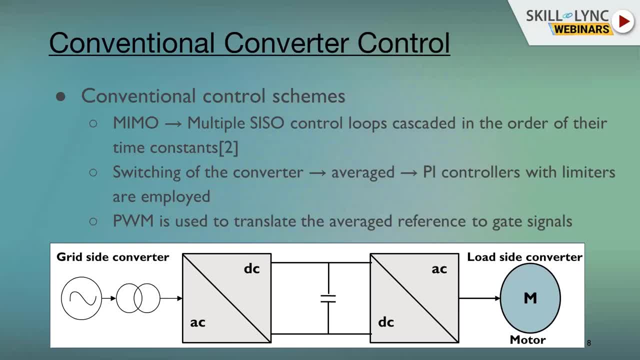 which is, of course, which is very small in nature and normally neglected. So when we do such kind of control or when we look at the system in that perspective, we normally tend to average the control. So PI controllers with limiters are naturally employed, by neglecting the switching action. 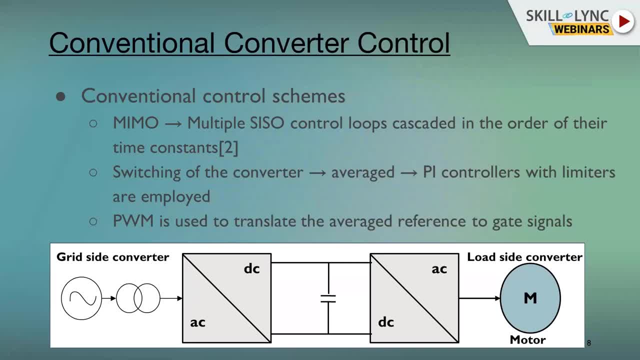 of the controllers Then, but again, the converters are discrete in nature. So a PWM modulator is used to translate this average reference into the gate signal by appropriately modulating. There are several modulating schemes. There are carrier based modulators. 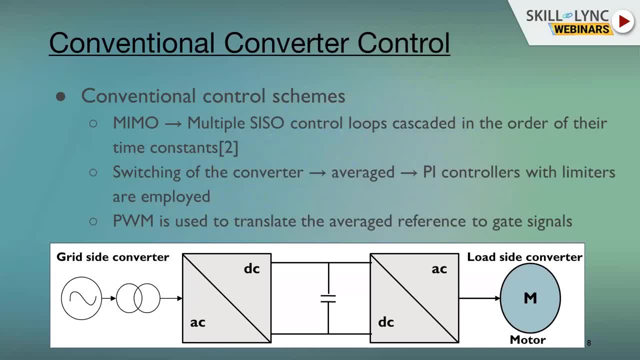 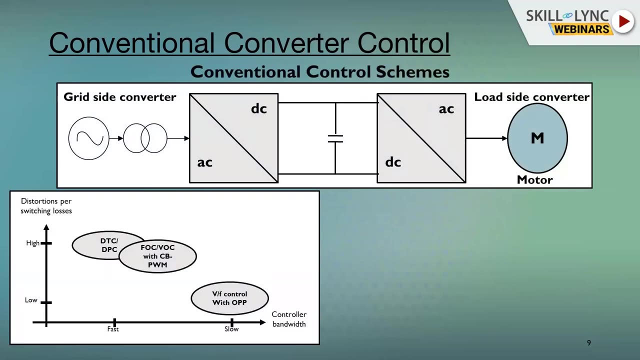 There are carrier based modulators. There are carrier based modulators And there are space vector kind of modulation schemes that are available in the literature. So, but typically for all the conventional control methods, these three are the major attributes. Having said that, where do we stand with the conventional methods? 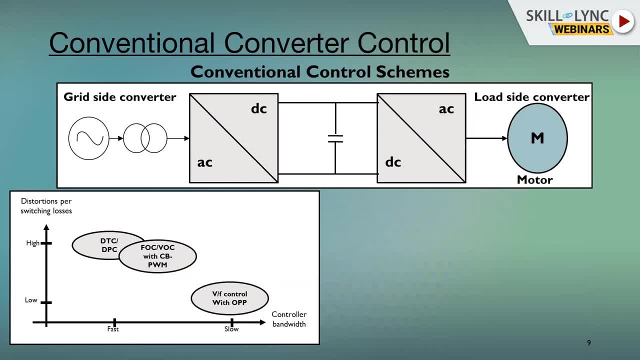 So if we see the conventional methods, the DTC and DPC are very good in giving a fast, dynamic response, but their harmonic distortions and switching losses are little higher, Whereas the optimal pulse pattern control, which can give you low distortions, but they 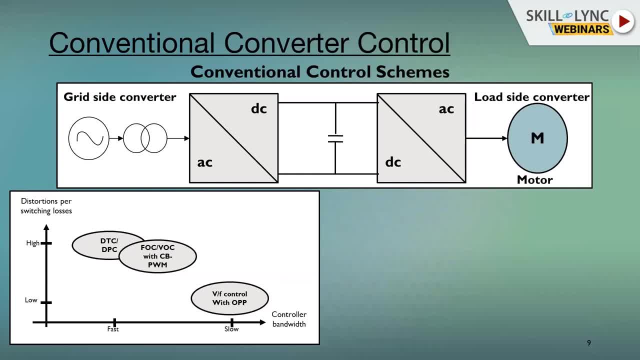 can't be used for a higher bandwidth controller Like their speed of response is not that good. Now FOC and VOC. with carrier based PWMs they fall somewhere in between, but substantially the distortions are little higher but you can get reasonably good speeds. 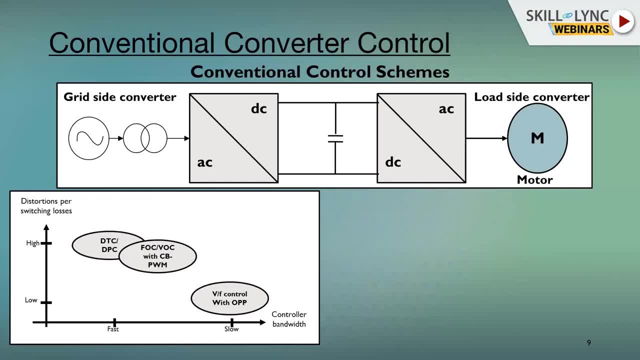 Now, If at all, if there is a method or an algorithm that actually combines the positives of these two, like a method that can operate in the region that is lower or that is closer to the origin of this plot, it would have been much better. 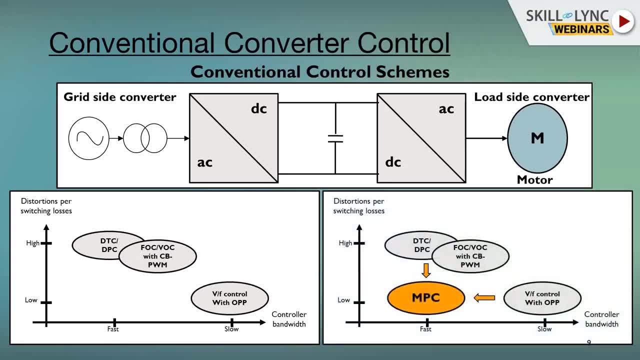 And fortunately model predictive control algorithms really fall into that category, wherein we can get low distortions per switching losses and at the same time a fast response similar to direction. So model predictive control is a combination of the advantages that direct or control or 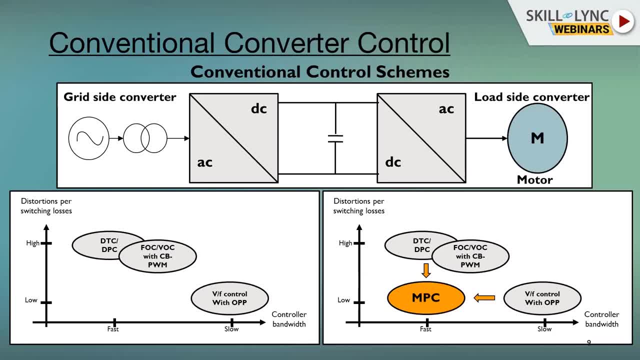 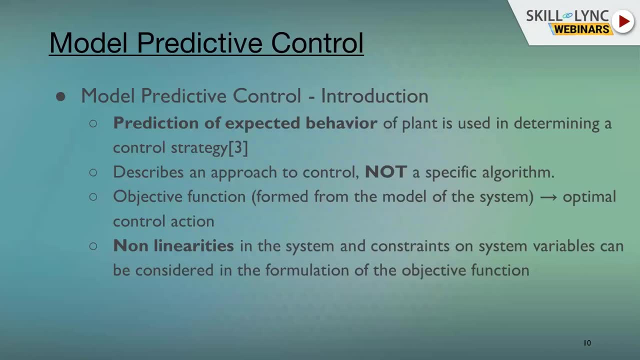 direct power control offers, along with the optimum pulse, but the advantage of low, low distortion that is offered by the optimal pulse pattern control. how this is happening We'll be seeing in the subsequent slides. So what is model predictive control? So typically, 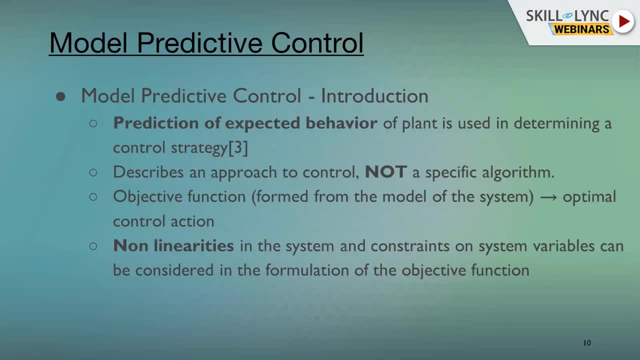 The model predictive control algorithms. they have their existence in from 1960s, but they are mainly used in process control rather than electrical control of power electronics. The control of power electronics model predictive control only picked up in the very recently, in the recent decade, wherein, with the advent of high speed digital controllers, 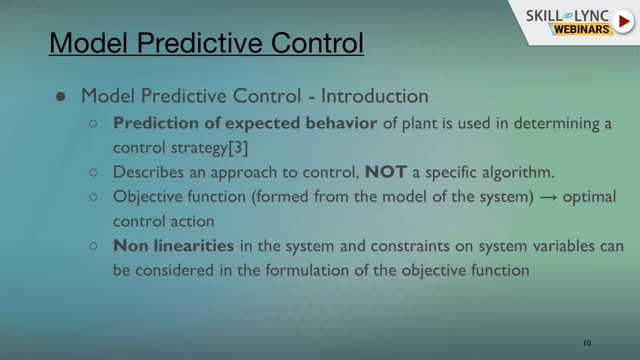 So what does actually a model predictive control says? typically, model predictive control uses a prediction of expected behavior of plant. as the name suggests, We tend to predict the behavior of the plant and determine an appropriate control strategy. Now the most important point or important feature of model predictive control is: it is a control. 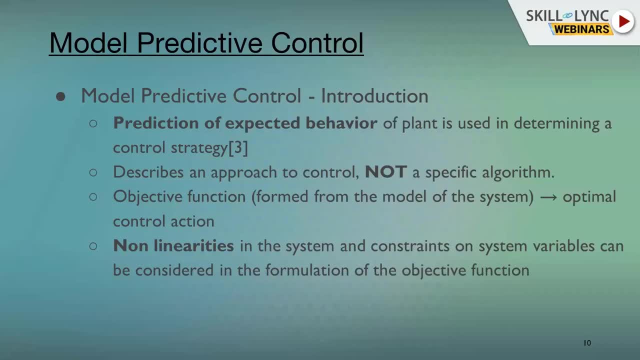 philosophy rather than a specific algorithm. The idea is what the model predictive control gives. It is not a specific algorithm. There are too many formulations, There are too many Uh understandings of this, but the philosophy remains the same, but there can be many ways of implementation. 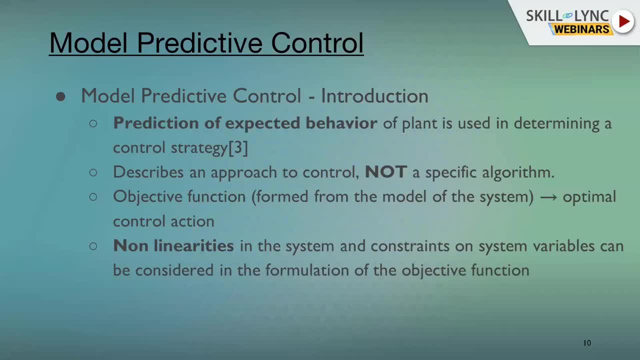 Now, another advantage is we have an objective function again that can be formed or formulated from the model of the system, and the objective function can be designed such a way that, directly from the objective function, we may arrive at an optimum control action in the, in controlling the system. 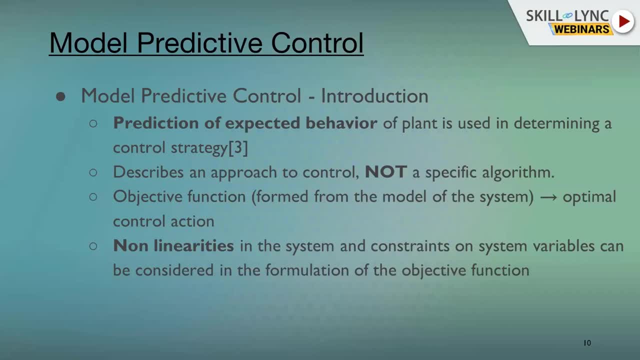 Now, another typical feature of this control philosophy is if there are There are nonlinearities in the system, which are typically. any physical system has nonidealities and nonlinearities and constraints on system variables. They can also be directly considered in the formulation of the objective function. 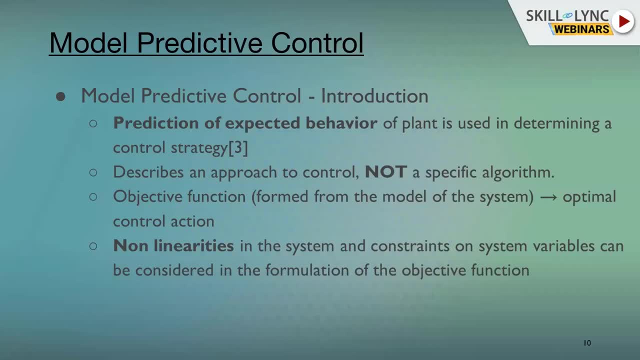 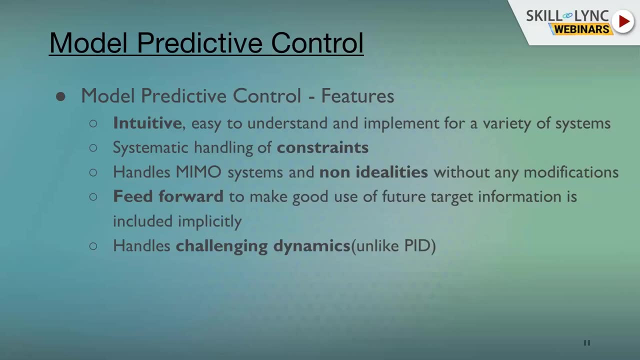 These are the main features or the main ideologies of model predictive control. Now, why is? why? is it why the model predictive control is more common or more prominent in the field of parallel? Now, it has certain advantages, or salient features, which are. the first one is: it is very intuitive, so it is very easy to understand. and if you understand the and implement for a variety of systems, 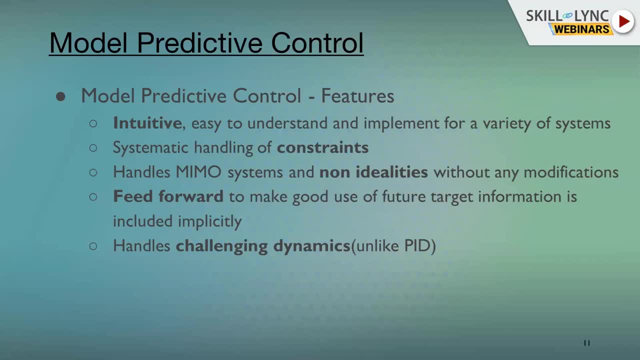 So if you understand the control philosophy for a single converter, you can extend it to any converter, or you can extend, and you can understand or you can extend it to any any converter that is available and provided you can appropriately model the Converter: Converter. 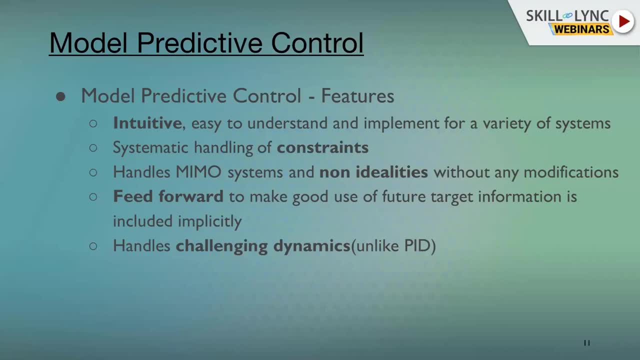 Now the constraints on the system, variables, whatever variables that you normally consider the, the constraints can be handled systematically. and then handles multi input, multi output systems and nonidealities without any Sorry, without any problems. then typically feed forward. it is also a feed, it is implicitly feed forward control. so there is a feed forward control implicitly. 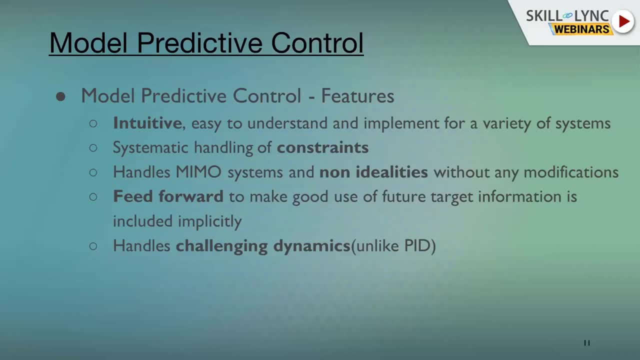 So there is a feed forward control implicitly Embedded in the control algorithm itself, So you can get a. you can get a very good control response, a combination of feedback and feed forward controls and and and. unlike PID control or any conventional PI based control model, predictive control can handle challenging dynamics. 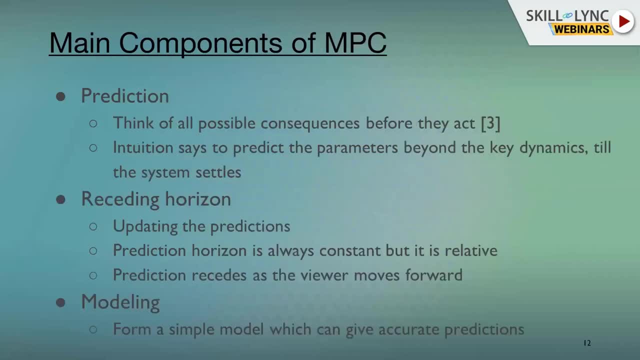 So let us go to what are the main components are. rather, I would say these are main stages in implementation of a model predictive control. the first stage is a prediction. the prediction is something like, as the name suggests, you have to predict the future or predict the behavior of the system, so you have a control action for your controller. 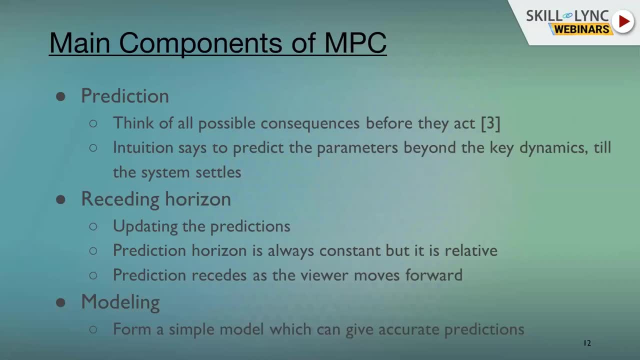 you try to predict the possible consequences. like, let's say, i have a control action. i try to put this control action onto the converter and see how the converter behaves now. what parameters are going to change. if you have a proper mathematical model, you can just predict the behavior or predict. 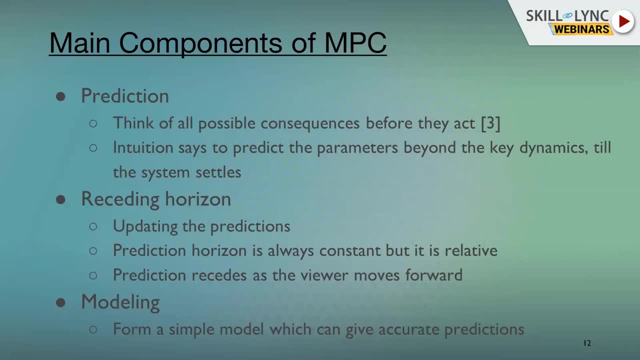 the parameters. now, while designing the prediction, you need to understand that you need to predict the change or the predict. let's say you give a control or you give a change in the control action. you need to predict the system till it settles. so that is one, one stage or one point that you 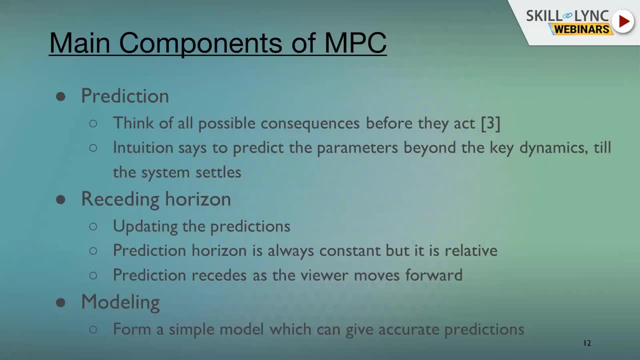 need to take care when you are predicting now. second one is receding horizon. receding horizon is something that deals with updating the predictions, so it is like how frequently you are updating, or it can also be thought as a moving window. like you are actually, you have a horizon, like you have a vision and you are constantly moving in time. 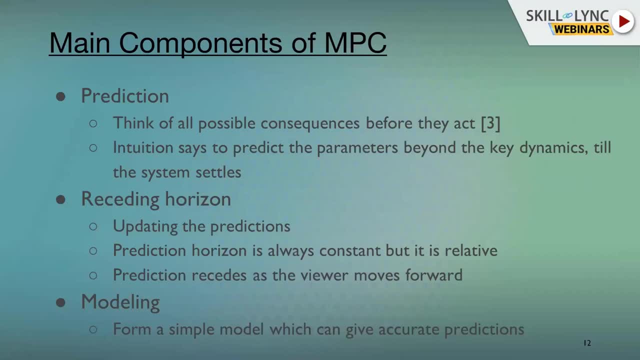 so as you go forward in time, your window also goes forward in time. so your past prediction- sorry, present prediction- becomes the past prediction. i mean for the future sample. so it is like you are predicting at this sample. the future value will become the present value for the next. 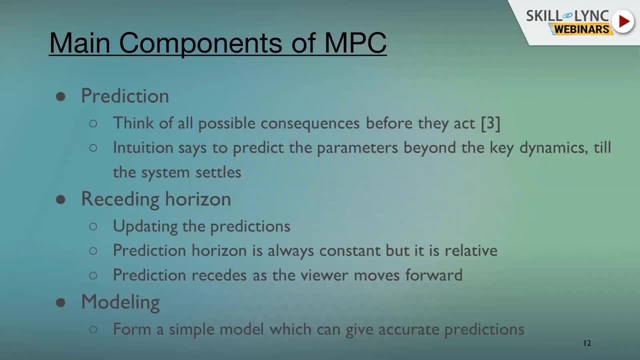 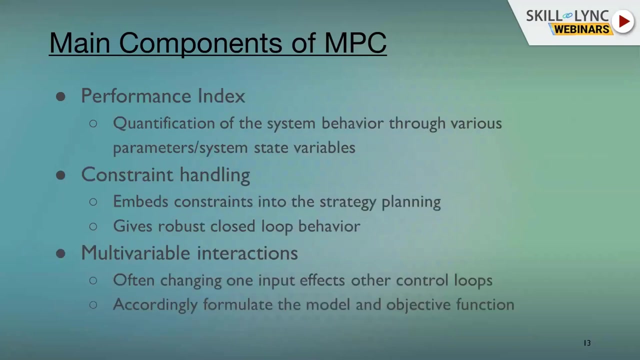 sample that how it goes. so that is what the prediction receives as the viewer moves forward. now modeling. modeling is another stage where you need to form the model of the system which can give recent decent, accurate predictions. and next stage, or next component, is performance index. so the 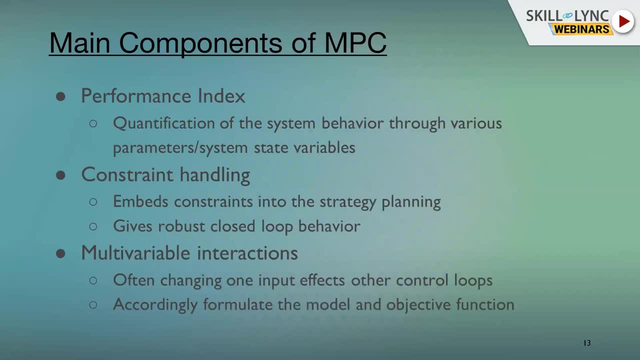 performance index. here is the quantification of system behavior. or let's say the performance index is a constraint or a value of a variable of the system. let's say i take. typically i take a current current in a power electronic converter. the thd on the current can be a performance index. 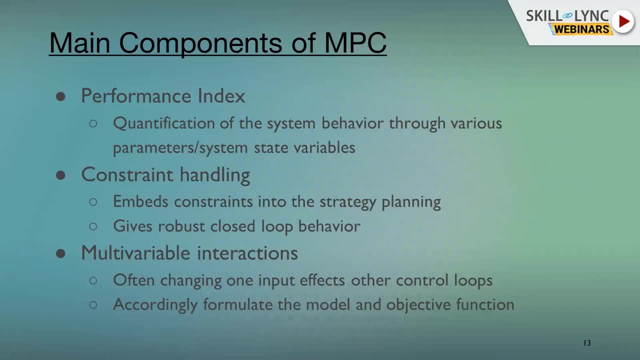 like you try to control the thd on the current to particular value, or you have a torque on a motor. you try to control the torque onto a particular value, or you try to uh, take the torque ripple and try to keep it in two bounds or something. so you need to frame. 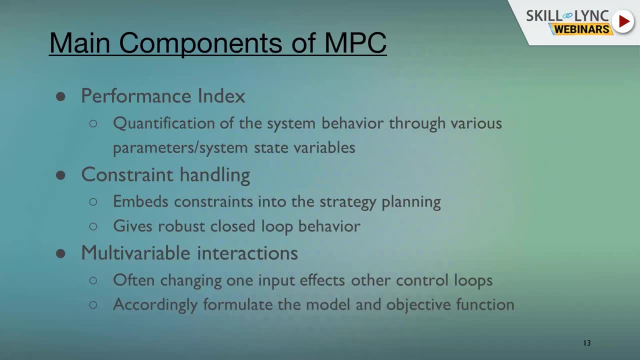 performance indices of your system and then formulate your control accordingly. then there are constraints. now how you are going to embed the constraints into the control philosophy or control methodology is another stage of implementation of a model predictive control. now constraints typically can be implemented in a power electronic converter, for example. let's say you want to have an over. 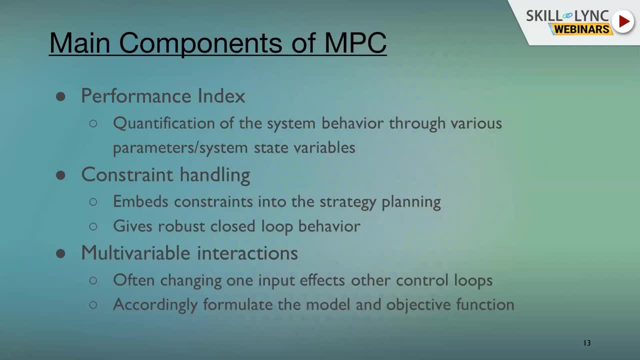 current protection. so you should, you should put a limit on the value of the current that you are getting. so that is, that in itself is a constraint. another example for that can be a common mode voltage on a example, a common mode voltage on a power converter, so that you may have different. 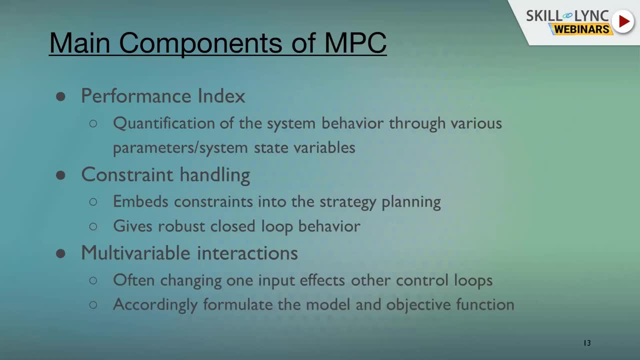 levels of common mode voltage on a power converter and you want to limit the or limit or reduce the common mode voltage, you can put that as a constraint. so this kind of constraints, when, when you put on the system or when you embed into your problem formulation that gives a robust closed 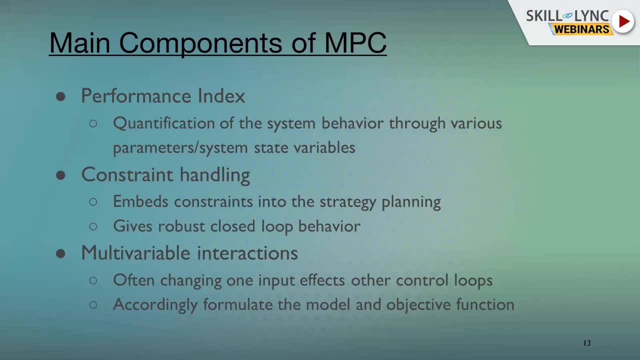 loop behavior. so usually in conventional control, the pi controllers. we have limits on the pi controllers just to make sure that the system will be within bounds. a similar, this constraint handling stage can be considered as a similar stage where you you have to make sure that the responses or the parameters that you are considering. 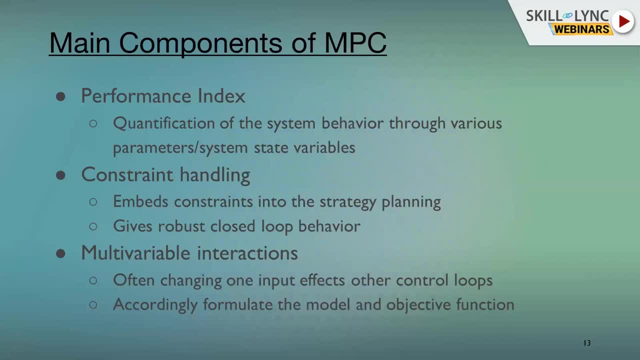 should not cross a value beyond. it should not go beyond some particular limiting values. then comes the multi-variable interactions. now often what happens in the physical systems? any physical system, a decoupled control is not at all possible, it is practically impossible, i would say. often when the input to one particular loop changes, that affects the 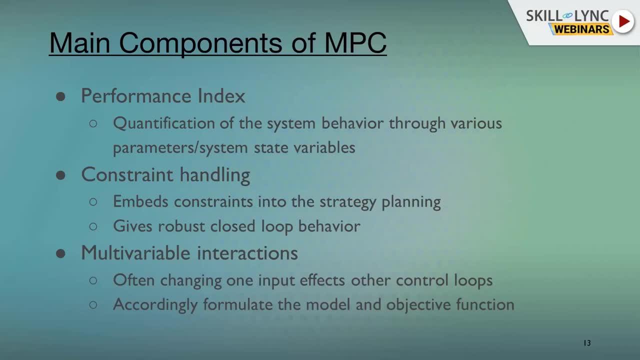 other loop as well, but typically in the conventional control methods we tend to ignore and we tend to go with the superposition principle wherein, when- all when- you are considering one input for a one output system, all the other inputs for the system are typically considered as disturbances and they are rejected. however, the physical systems may not be. 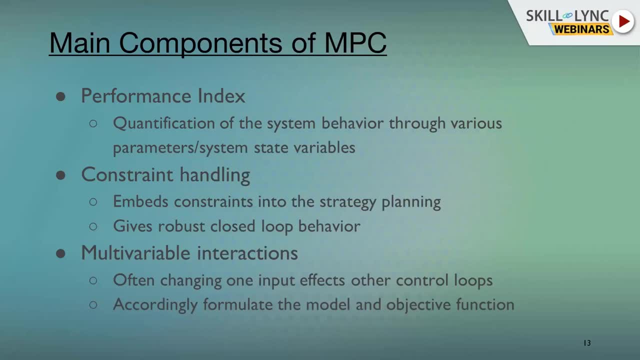 working like that. so how the multi-variable interactions that are happening are how the multi-variable interactions are happening in the system you need to understand. and then the objectives are, the model model and the objective function can be formulated. so these are the typical stages that one encounters in the design. 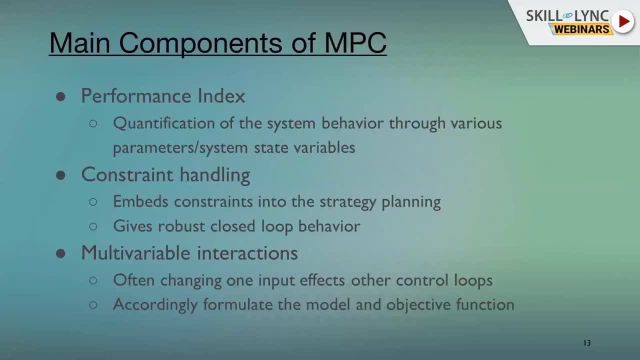 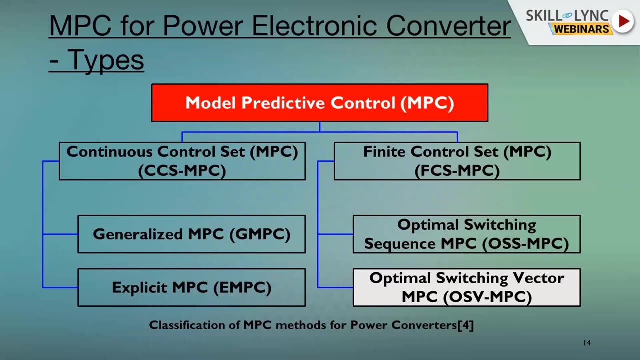 and implementation of a model predictive controller. now, moving on to what are the types of model predictive control schemes that are available for power electronic converters? broadly, there are two schemes that are available. one is continuous control set- mpc- and finite control set- mpc. so a continuous control set mpc is a continuousésmstudio, but something that either 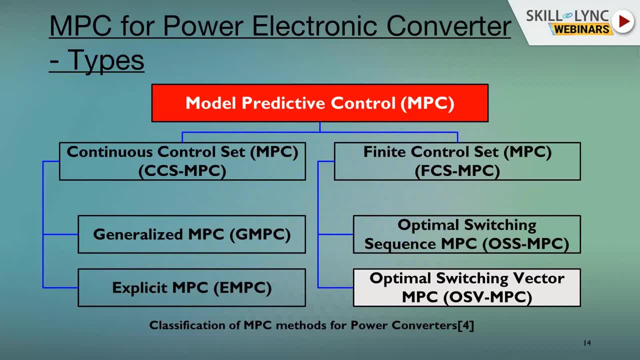 of these two is present. ok, so for pinky, perfect. simply, a continuous control is a continuous control, specially at mpc. the output of the controller is a voltage, a continuous signal, wherein you need to use a modulator to generate the gate pulses and control typical, typical.